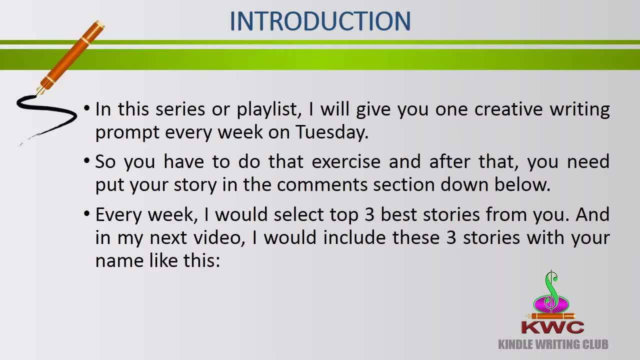 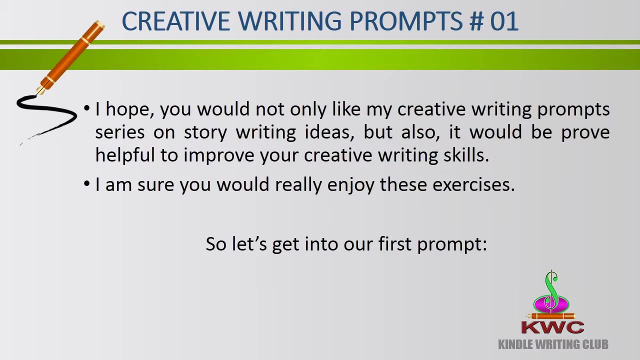 you need put your story in the comment section down below. Every week I would select top three best stories from you and in my next video I would include these three stories with your name. like this, Your written story will be shown here. I hope you would not only like my creative writing prompt series on story writing ideas. 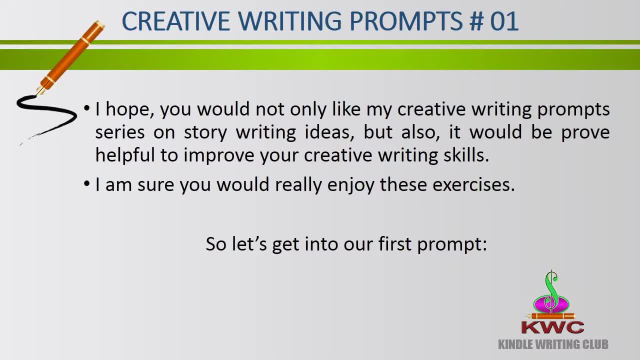 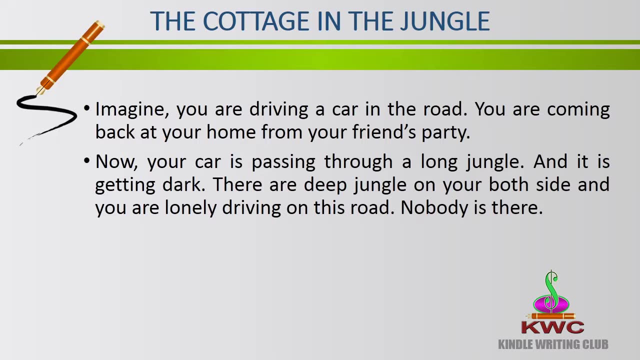 but also it would be prove helpful to improve your creative writing skills. I am sure you would really enjoy these exercise. So let's get into our first prompt. Imagine you are driving a car in the road You are coming back at your home from your friend's party. Now your car is passing through. 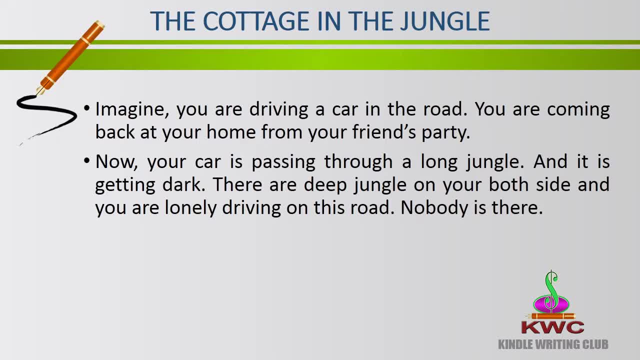 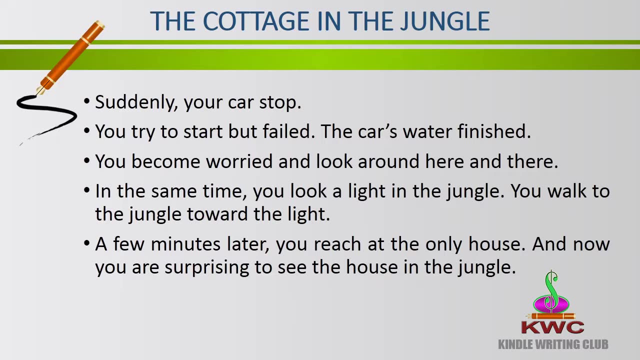 a long jungle and it is getting dark. There are deep jungle on your both side and you are lonely driving on this road. Nobody is there. Suddenly, your car stop. You try to start but fail. The cars were finished. You become worried and look around here and there In the same time. 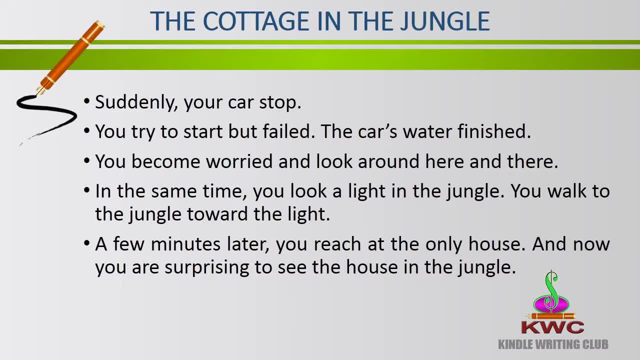 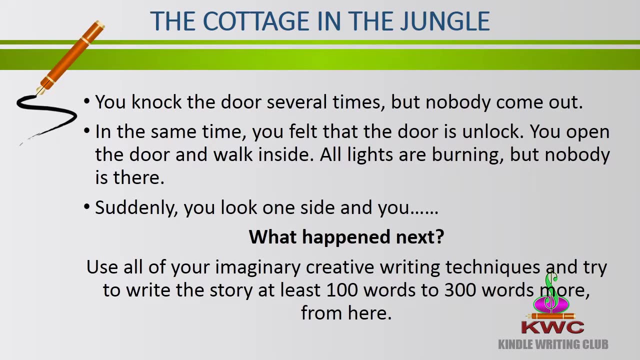 you look a light in the jungle. You walk to the jungle towards the light. A few minutes later you reach at the lonely house And now you are surprising to see the house in the jungle. You knock the door several times, But 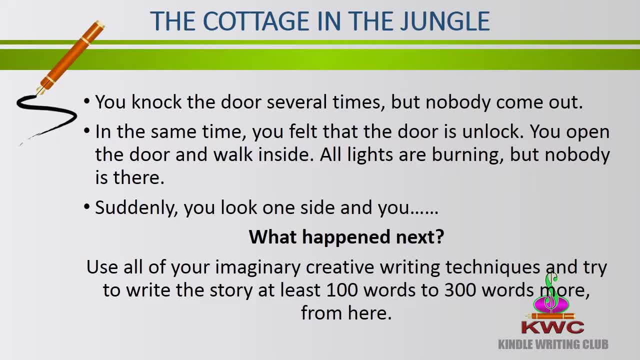 nobody comes out. In the same time, you felt that the door is unlocked. You open the door and walk inside. All lights are burning, but nobody is there. Suddenly, you look one side and you… What happened next? Use all of your imaginary creative writing techniques.